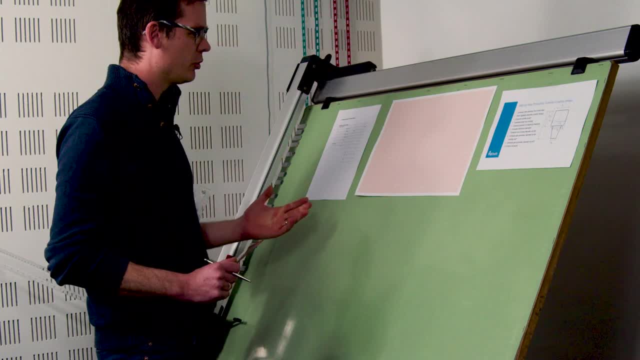 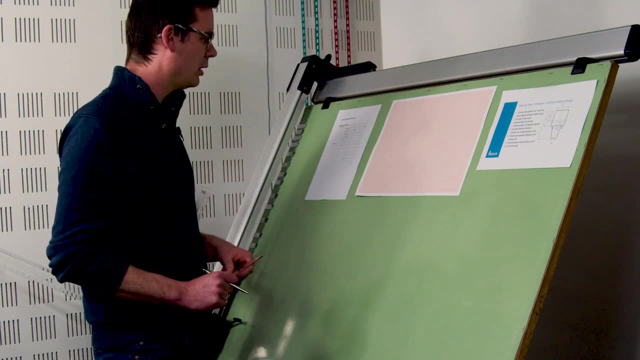 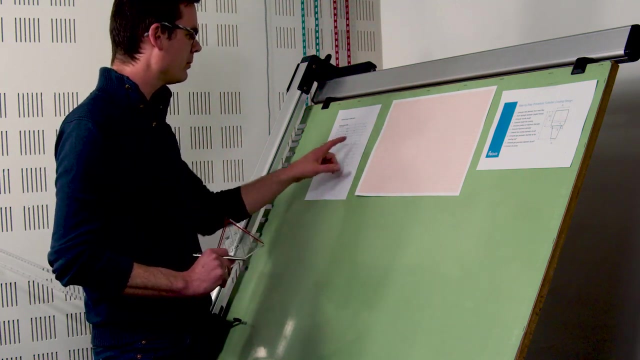 that cowling Alright. the first thing we need to determine is the scale. I have an A3 paper here. If I look at the length of the turbofan engine, the whole cowling length is 7 meters and 10 centimeters in my calculations. So I'm deciding to use a. 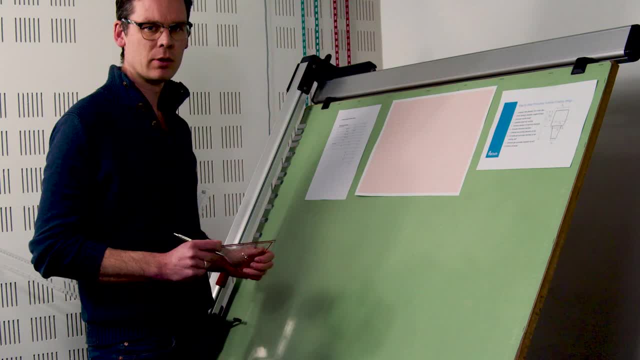 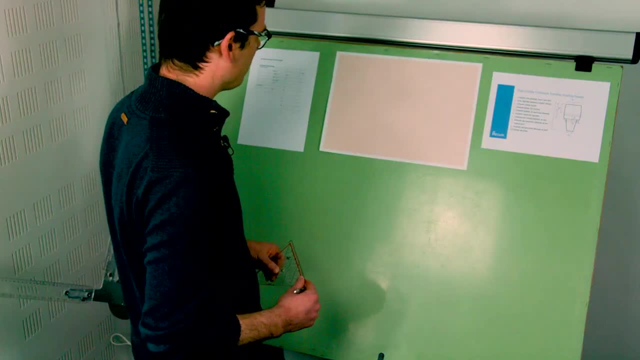 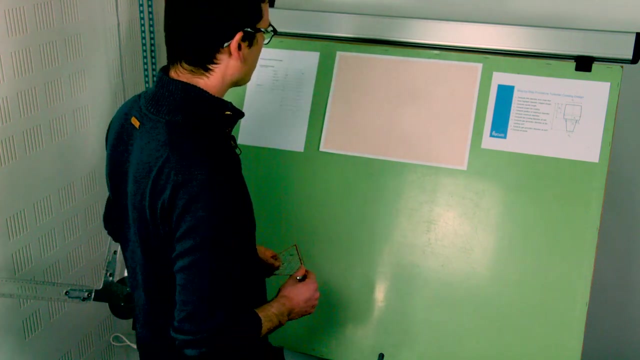 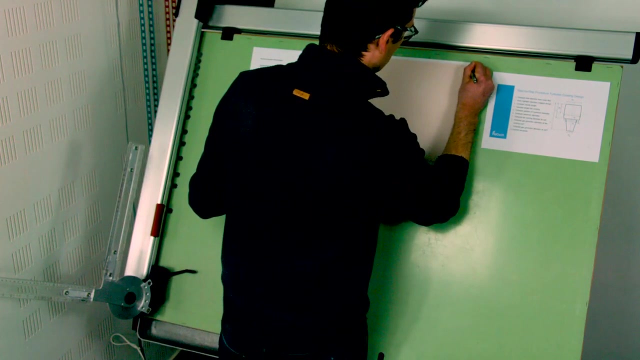 scale 1 to 25 to draw this engine, such that you get a nice large engine on this, on this sheet of paper. Now we're going to draw both the top view of the engine, or side view, as it is actually symmetric, As well as part of the of the front view. So I'm writing down the scale for future. 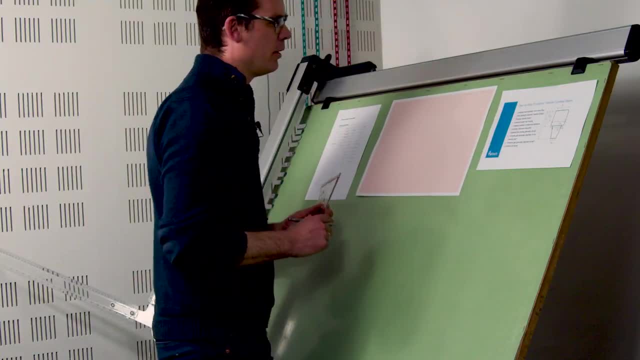 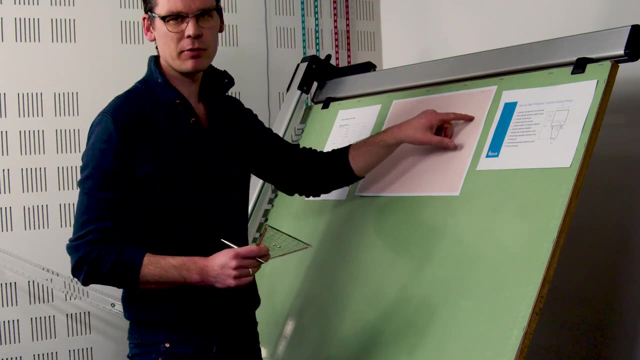 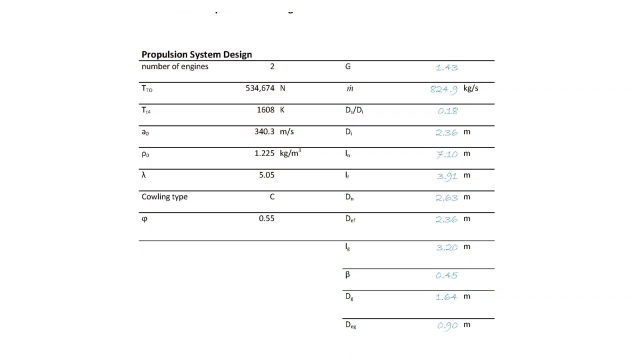 reference 1 to 25. and the first thing I'm going to do is again draw the, the reference center line of the engine. And I'm looking at my my data sheet here. I'm seeing that the diameter of the engine, maximum diameter, is 2.6 mm. 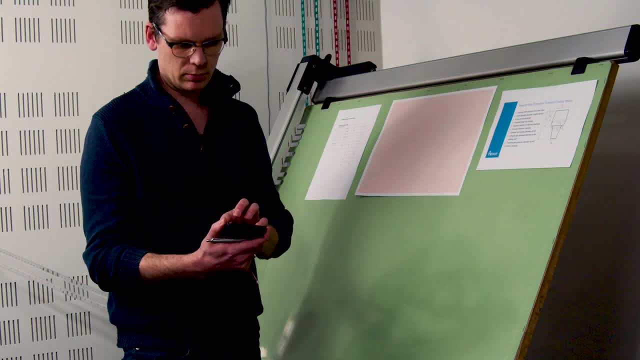 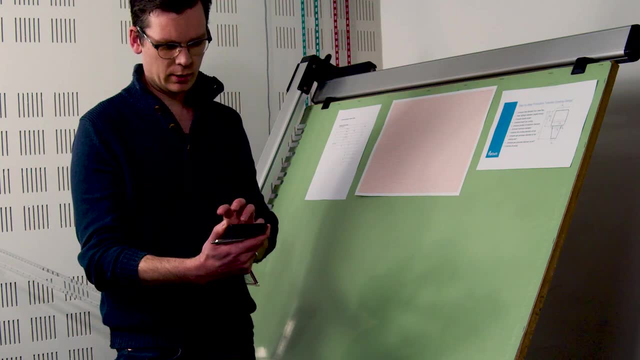 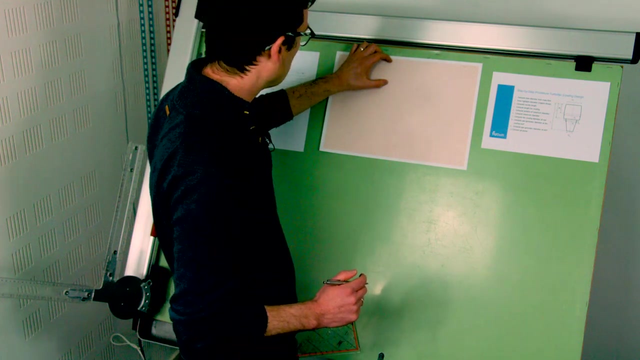 So 2.6 Window, pretty dry 0.25торов. divided by 2 is beaxle 5.26 centimeters, Which is gonna be the radius on on the drawing. So I'm making sure that I'm at least, let's say, 7 centimeters off of the top to draw my, my central line to. 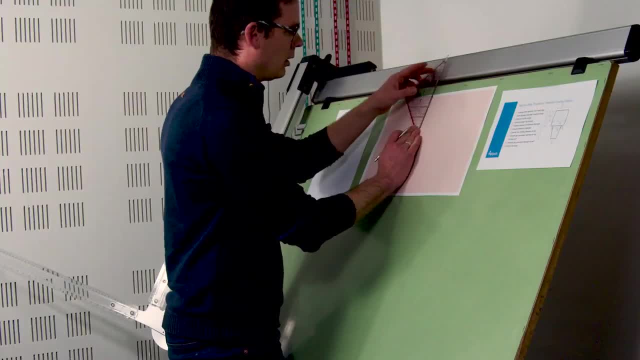 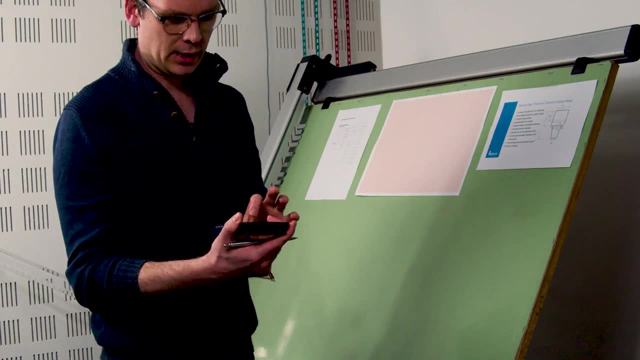 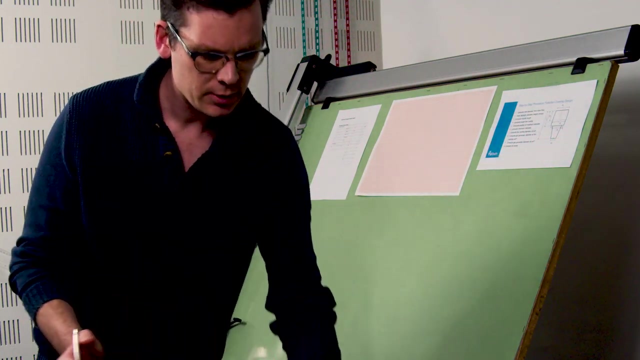 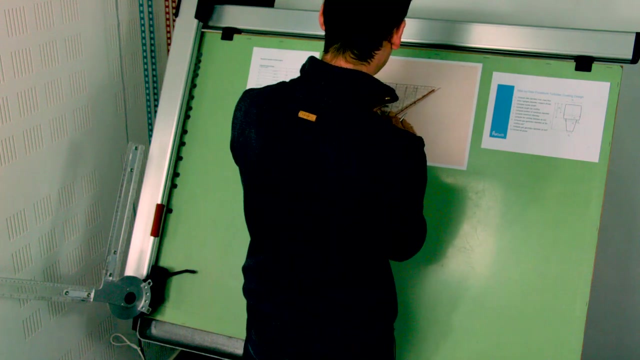 give me some nice space. So 7 centimeters off of the top ahead there, and I said 7 meter, 10 is the length, 7.1 divided by 0.25 is 28 centimeters. well, my protractor is about 22, so 22 plus 6 give me approximately. 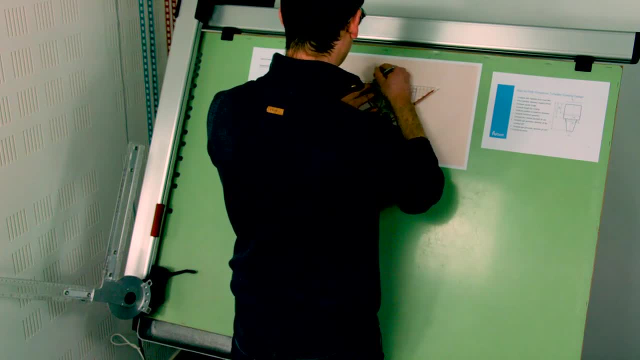 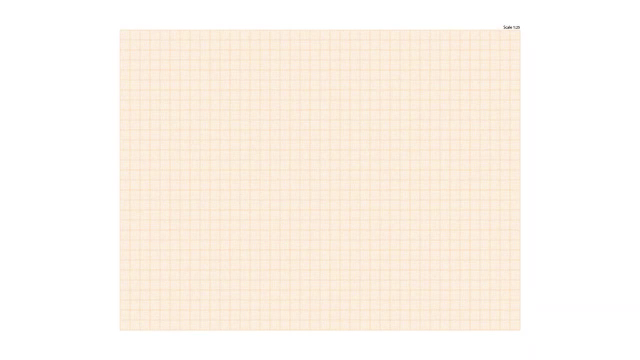 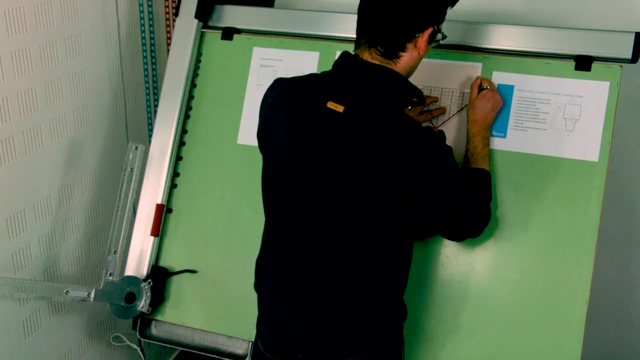 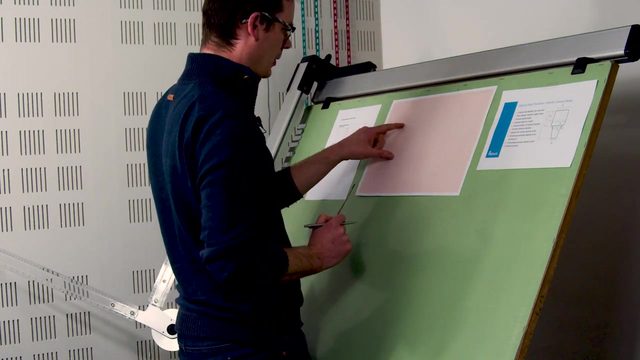 starting point over here. I'm gonna add another centimeter, so I'm gonna start roughly over there. so first draw my symmetry line here as a dashed dotted line, and it's gonna be the line that I'm gonna use throughout the rest of the drawing, right? so I just said the diameter is going to be approximately. 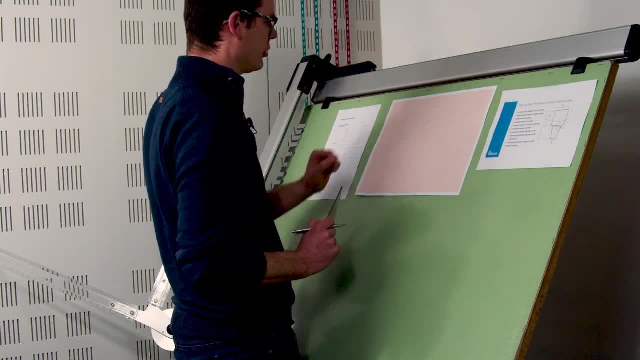 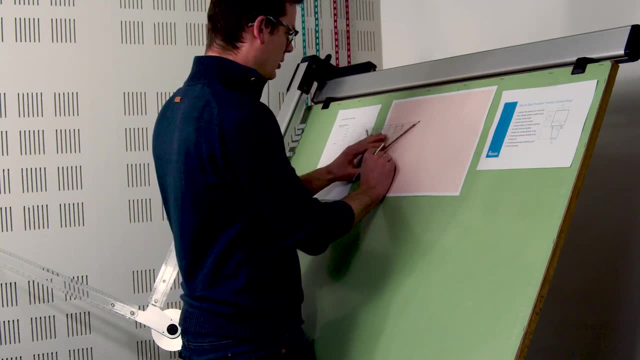 five centimeters, maybe a little bit more, on this on the sheet. so if I want to draw here a complete circle, I might not be able to fully do that. give me some space here. I'm just gonna make part of a circle and I'm putting the center line over here, and that's okay because it's 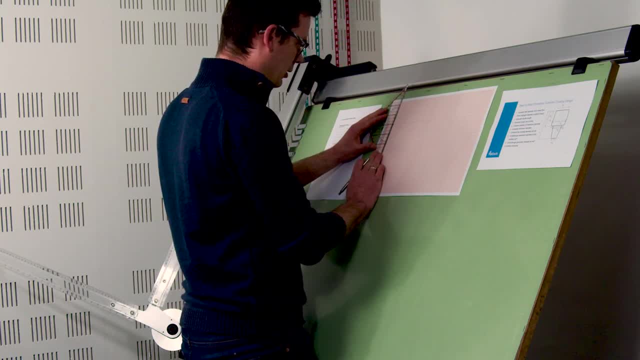 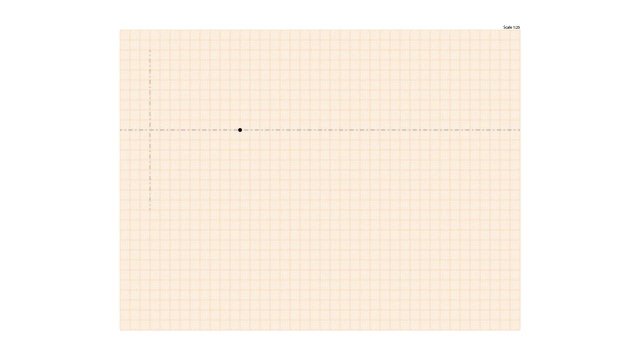 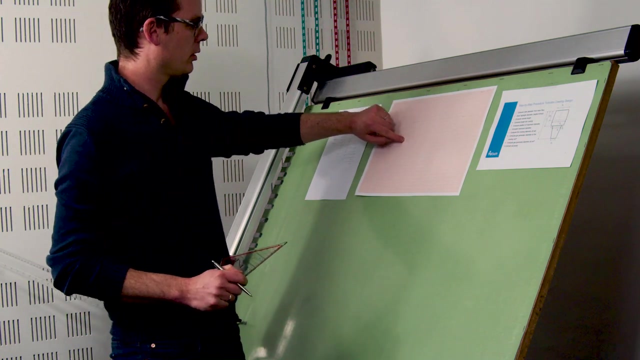 actually symmetric anyway. so if I draw even half of being at the of the front view, you can already understand what it looks like in front of me. so I'm gonna fill right. so the next thing I'm going to do is I'm drawing, drawing the the. 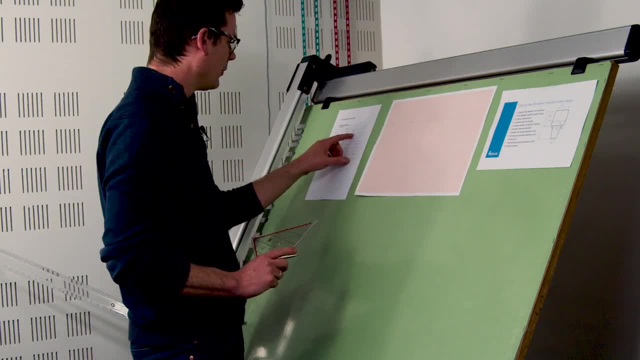 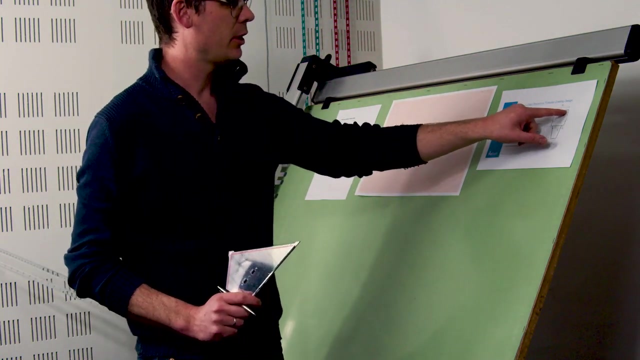 highlight face of the turbo fan. I'm assuming here that the highlight and in the inlet have the same diameter, so that the inlet diameter is 2.36 meters. that has been computed and I'm assuming the highlight diameter is exactly the same, the highlight diameter indicated on the sheet here, so 2.36 divided by 0.25 and 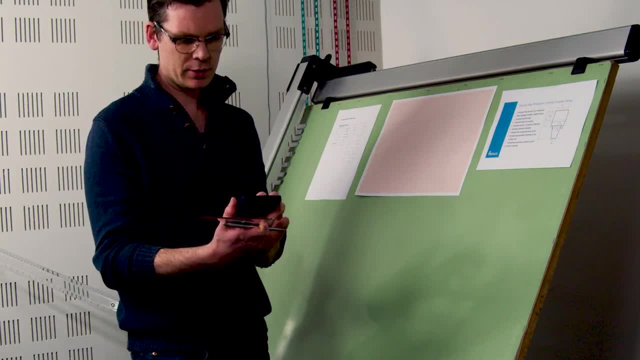 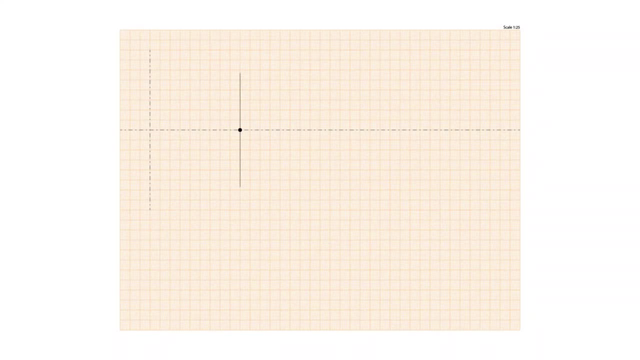 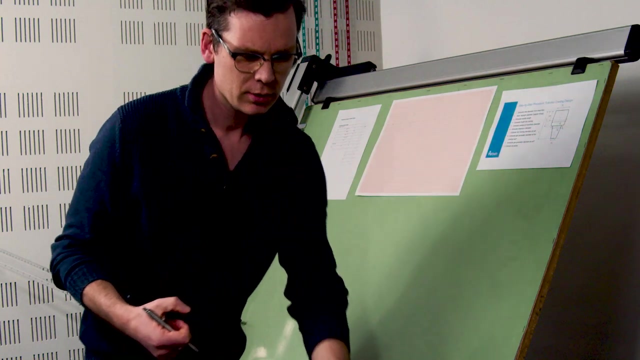 9.44 is the diameter in terms of centimeters. divided by 2 gives me a radius of 4.7 centimeters. so this is my inlet face. next thing maybe is to to draw the end of that engine. so it was 7 meters, 7.10 meters, I think I did the. 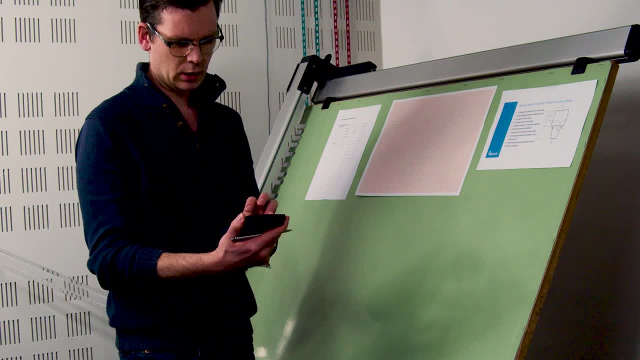 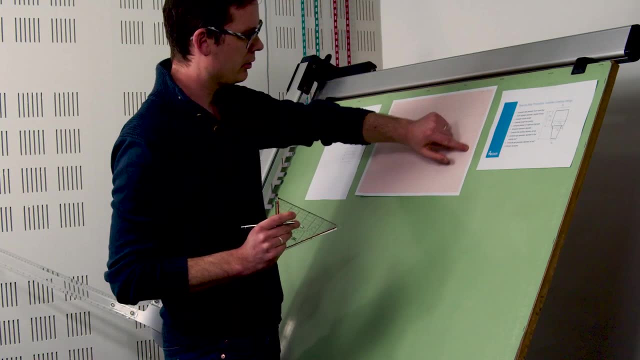 calculation already, but let's do it again. 28.4 centimeters gives me a point over there. I'm gonna later on show you how to do that. so I'm gonna draw a point over there. I'm gonna later on show you how to do that, so I'm gonna later. 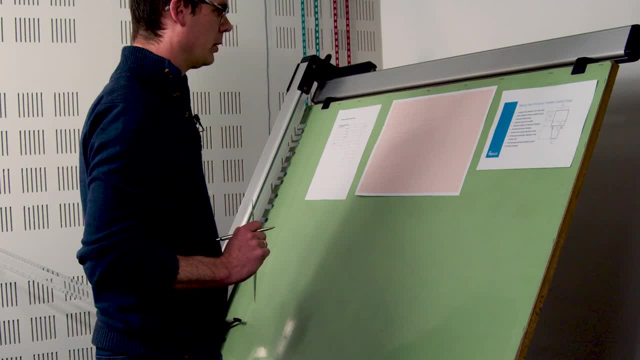 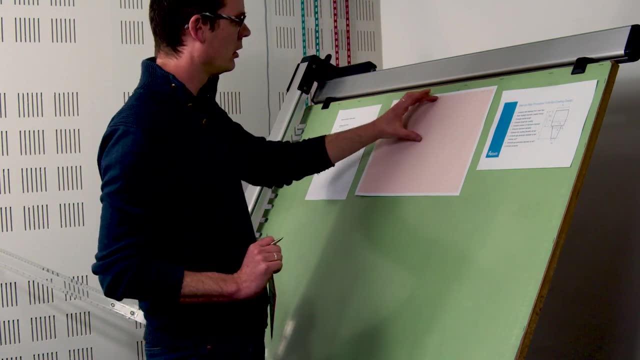 on extend that, but for now I know this is where my engine is going to be all. on extend that, but for now I know this is where my engine is going to be all right. next point is to find the thickest part on the, on the cowling, which is the. 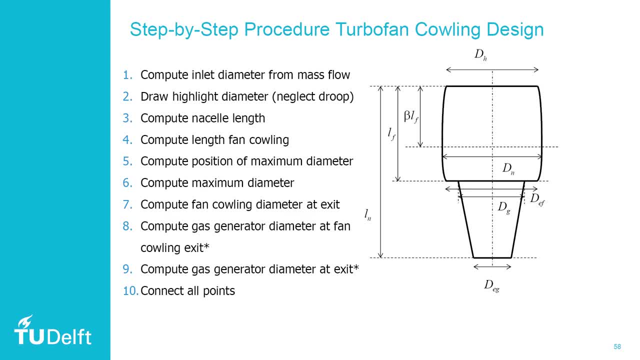 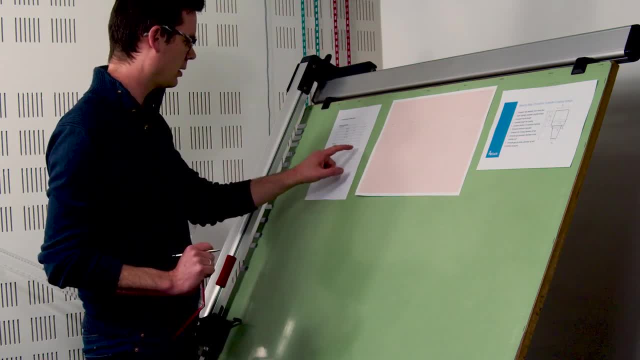 coefficient beta multiplied by the length of the of the fan. well, beta is 0.45. that's a decision that you make. it's a chosen value and the length of 0.45. that's a decision that you make. it's a chosen value and the length of the. 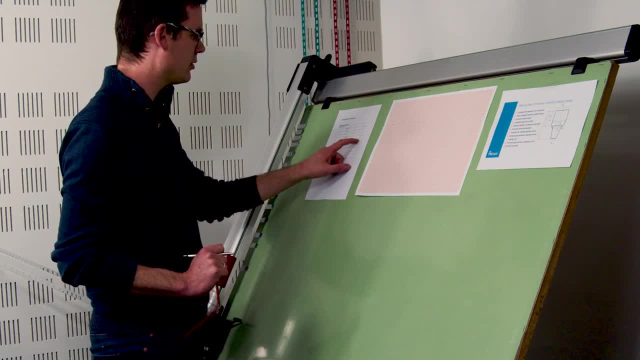 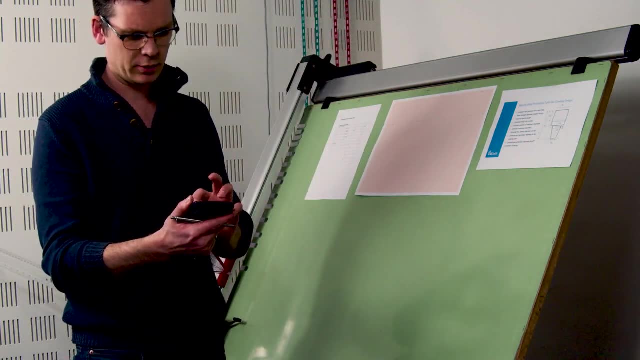 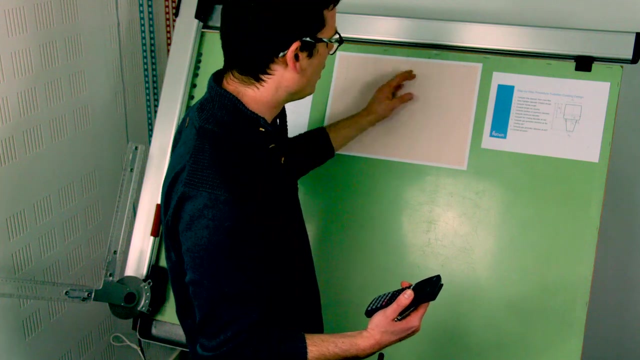 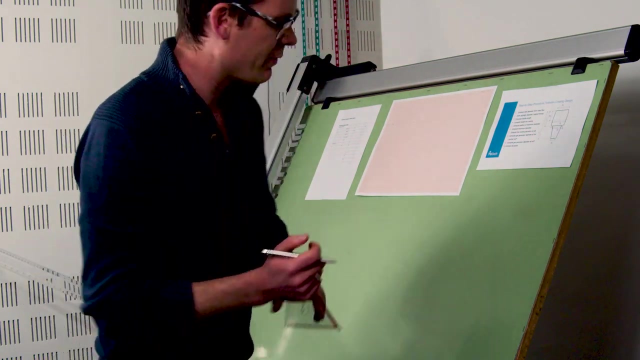 the length of the of the fan cowling is 3.91 centimeters. so if I multiply that 0.45 times 3.91 equals 1.76 meters from the inlet phase. I find the the largest diameter in there. so divided by 0.25 is set exactly 7 centimeters from the. 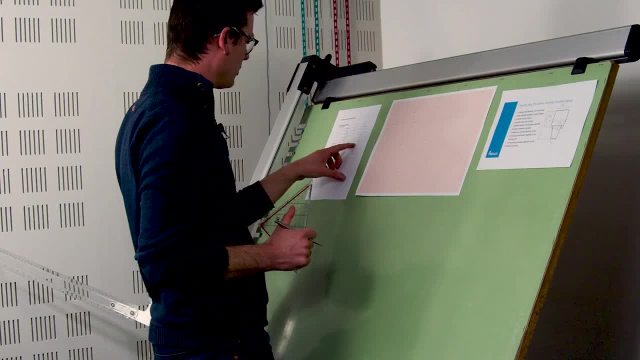 0.25 is set exactly 7 centimeters from the, the inlet phase, and then the maximum, the inlet phase, and then the maximum, the inlet phase, and then the maximum diameter. we, we said we computed this 2.63 diameter. we, we said we computed this 2.63. 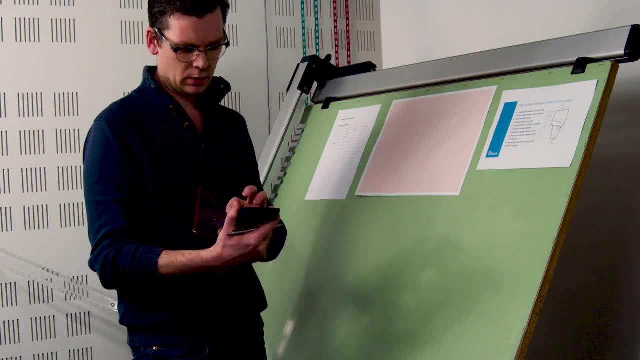 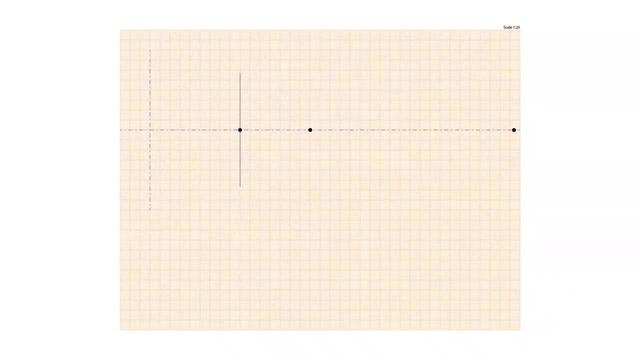 diameter. we, we said we computed this: 2.63 meters, which gives me a radius on the meters, which gives me a radius on the meters, which gives me a radius on the drawing of 5.3. and I'm just drawing a drawing of 5.3 and I'm just drawing a. 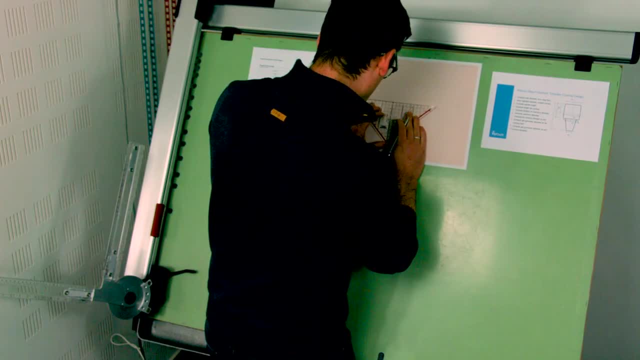 drawing of 5.3. and I'm just drawing a little straight line there because I little straight line there, because I little straight line there, because I know that is roughly what the shapes gonna know, that is roughly what the shapes gonna know, that is roughly what the shapes gonna look like over there, look like over. 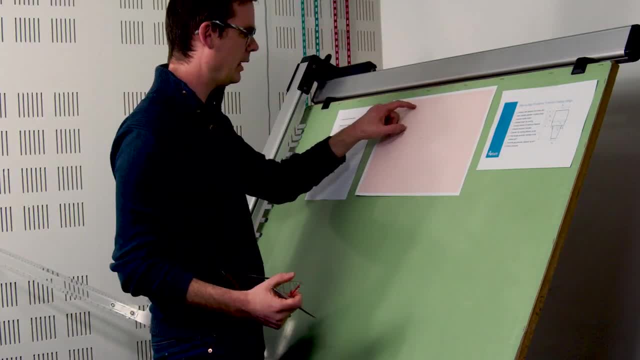 look like over there. look like over there. look like over there. all right, so I got my thickest point and all right, so I got my thickest point and all right, so I got my thickest point and got my inlet. next thing that I want to: 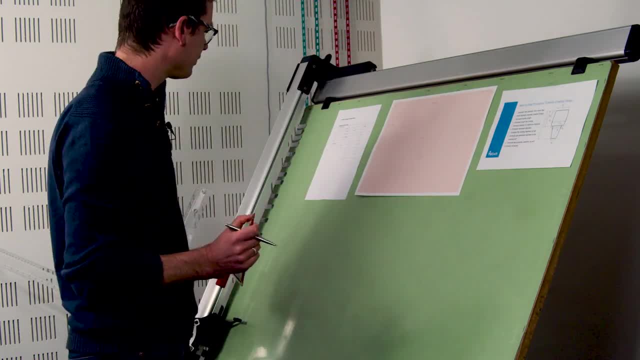 got my inlet. next thing that I want to got my inlet. next thing that I want to do is draw the rear part of the fan. do is draw the rear part of the fan. do is draw the rear part of the fan cowling so the exit of the fan: 2 meters. 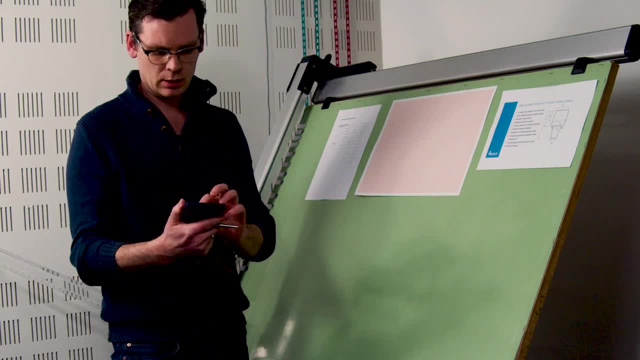 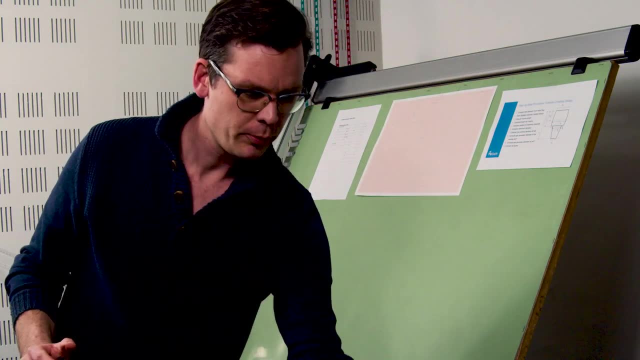 cowling, so the exit of the fan: 2 meters. cowling, so the exit of the fan: 2 meters. 36 centimeters in in real dimensions. 36 centimeters in in real dimensions. 36 centimeters in in real dimensions divided by 0.25 gives me a 4.7. 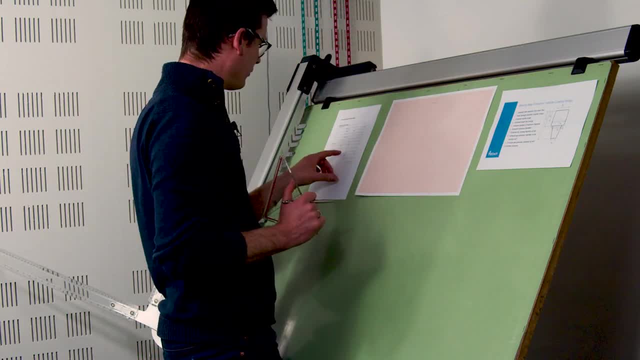 divided by 0.25 gives me a 4.7. divided by 0.25 gives me a 4.7 centimeter radius. okay, hold on, I first centimeter radius. okay, hold on, I first centimeter radius. okay, hold on. I first need to plot where the length of the fan. 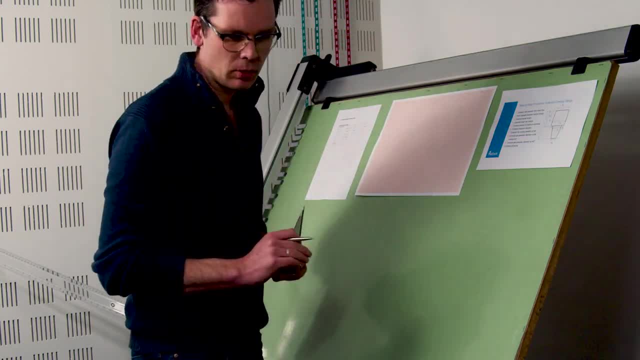 need to plot where the length of the fan, need to plot where the length of the fan, where the fan cowling actually ends and where the fan cowling actually ends and where the fan cowling actually ends, and that's so. I'm keeping in mind the 4.7. 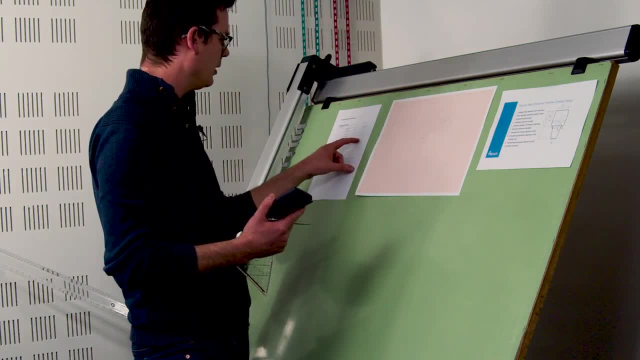 that's so. I'm keeping in mind the 4.7. that's so. I'm keeping in mind the 4.7 centimeters. and now I'm looking at the centimeters. and now I'm looking at the centimeters, and now I'm looking at the length of the fan counting, which is 3.91. 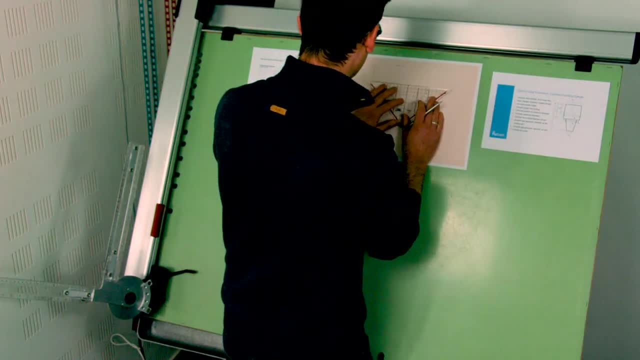 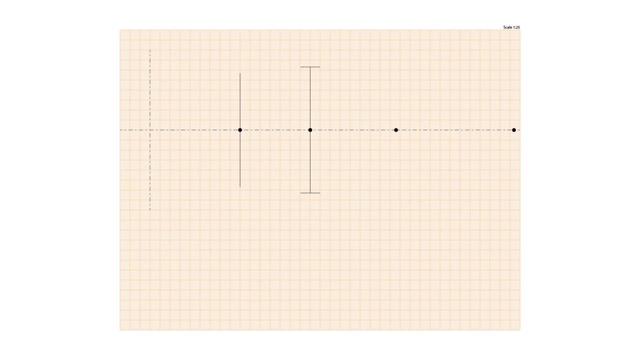 length of the fan counting, which is 3.91. length of the fan counting, which is 3.91. so after 15.6 centimeters, my fan. so after 15.6 centimeters, my fan. so after 15.6 centimeters, my fan cowling ends, I had a. 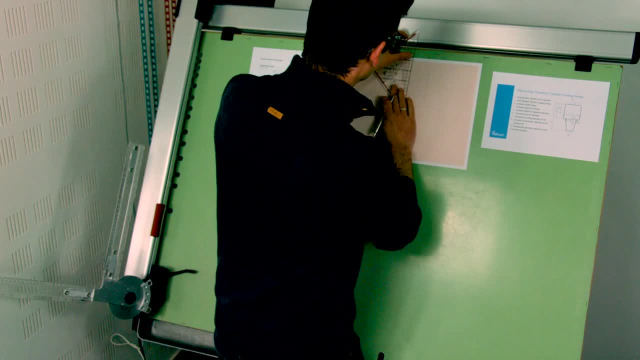 cowling ends. I had a cowling ends. I had a radius of 4.7 centimeters right, so I now radius of 4.7 centimeters right. so I now radius of 4.7 centimeters right. so I now have the exit of the fan cowling the. 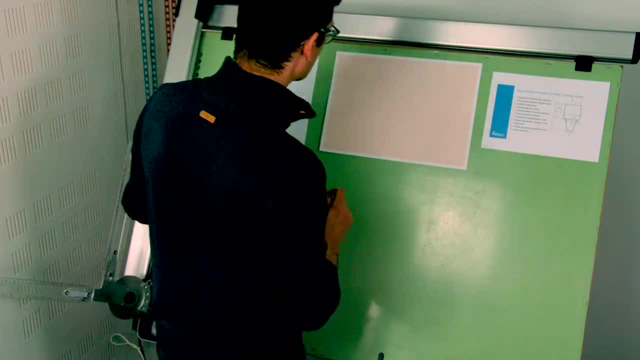 have the exit of the fan cowling, the have the exit of the fan cowling, the inlet of the fan cowling and the two inlet of the fan cowling and the two inlet of the fan cowling and the two outer points, and now it's sort of a. 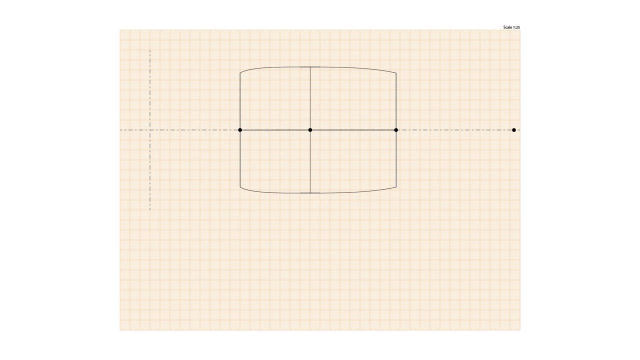 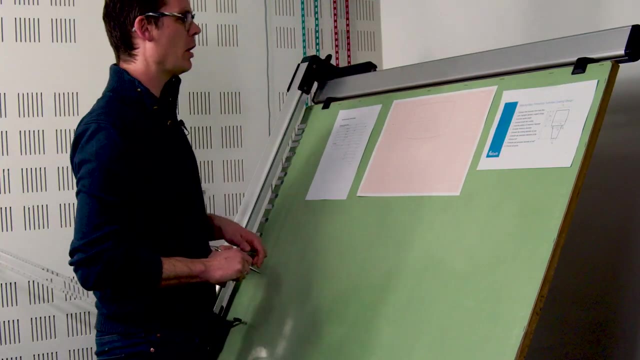 outer points, and now it's sort of a outer points and now it's sort of a connect the dots, connect the dots, connect the dots. so now we have the fan cowling done, and so now we have the fan cowling done. and so now we have the fan cowling done, and now we want to draw the cowling around. 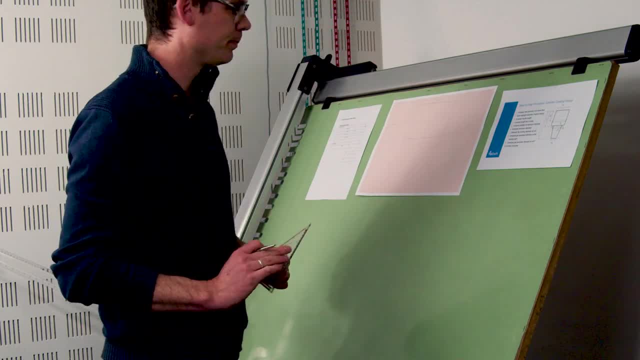 now we want to draw the cowling around. now we want to draw the cowling around the, the, the, the, the, the gas generator. so the first thing, gas generator. so the first thing gas generator. so the first thing that we do is we look at the, the gas. 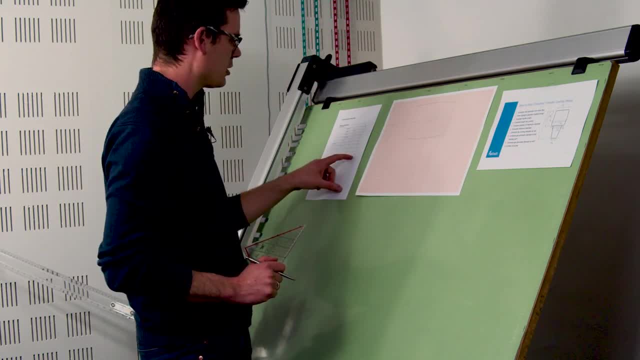 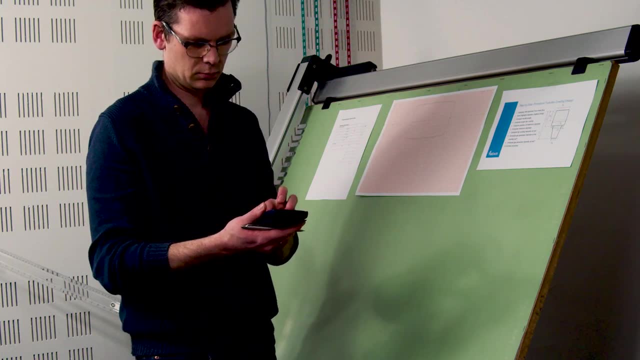 that we do is we look at the, the gas that we do, is we look at the, the gas generator diameter at the beginning. which generator diameter at the beginning, which generator diameter at the beginning which it says here is 1.64 meters, 1.64 gives. 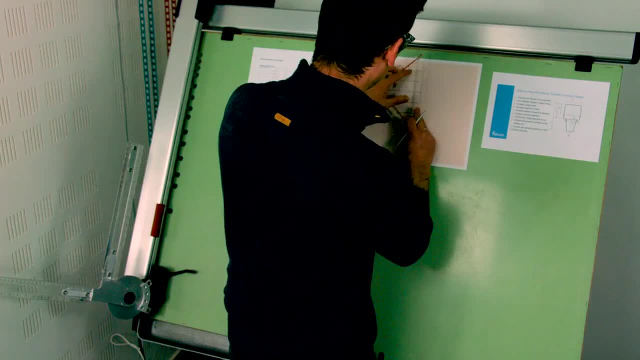 it says here is 1.64 meters, 1.64 gives. it says here is 1.64 meters, 1.64. gives me a radius on this drawing of 3.3 me, a radius on this drawing of 3.3 me, a radius on this drawing of 3.3 centimeters. 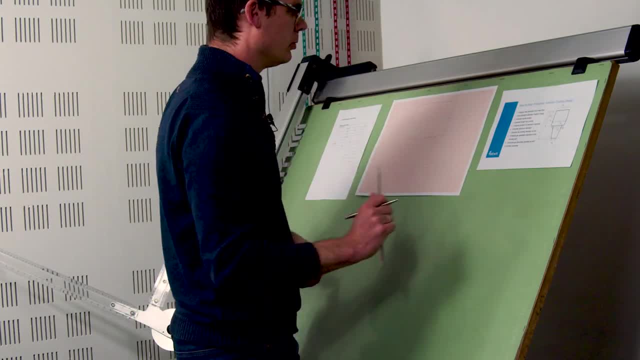 centimeters, centimeters, centimeters, centimeters. so that's the starting point, and now, just so. that's the starting point, and now, just so. that's the starting point, and now just need to compute the end of the gas. need to compute the end of the gas. 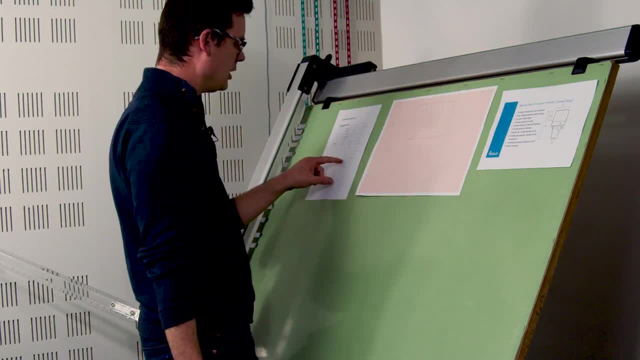 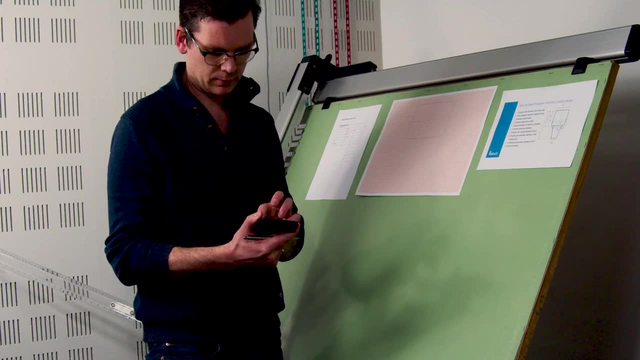 need to compute the end of the gas. generator it says deg is 0.9 meters. so generator it says deg is 0.9 meters. so generator it says deg is 0.9 meters. so 0.9 meters is 3.6 centimeters. is the. 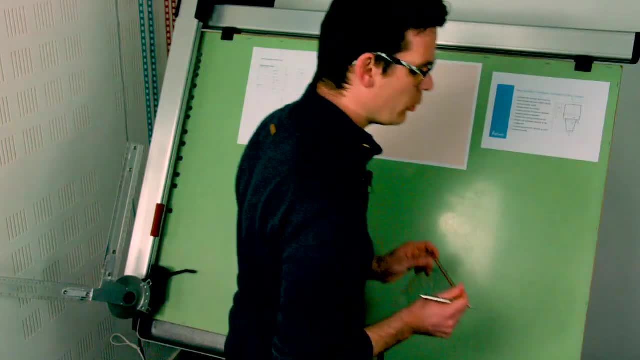 0.9 meters is 3.6 centimeters. is the 0.9 meters is 3.6 centimeters. is the diameter, which means a radius of 1.8 diameter, which means a radius of 1.8 diameter, which means a radius of 1.8 centimeters. on the drawing draw up: 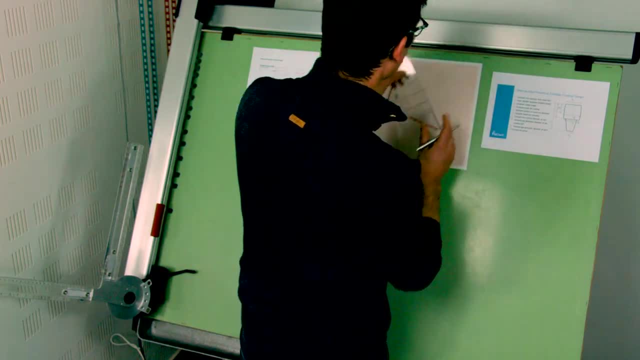 centimeters on the drawing, draw up centimeters on the drawing, draw up vertical line between those two, because vertical line between those two, because vertical line between those two, because that's actually the end of the gas, that's actually the end of the gas, that's actually the end of the gas generator cowling. and now I'm simply 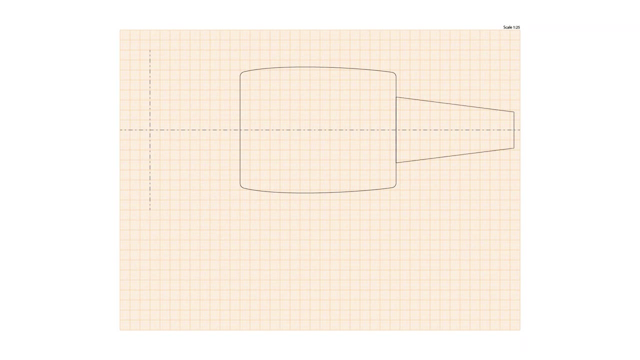 generator cowling. and now I'm simply generator cowling and now I'm simply connecting the dots with a straight, connecting the dots with a straight, connecting the dots with a straight line. and I have my gas generator cowling line and I have my gas generator cowling. 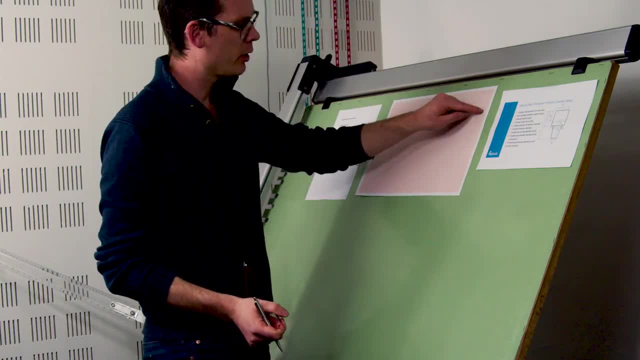 line and I have my gas generator cowling ready. note that we are not drawing the ready. note that we are not drawing the ready. note that we are not drawing the plug which is usually present at the rear plug, which is usually present at the rear plug, which is usually present at the rear end of the of the gas generator. we're 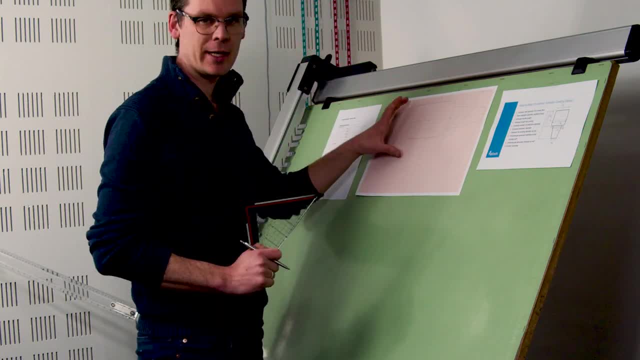 end of the of the gas generator. we're end of the of the of the gas generator. we're keeping that open for now. so this keeping that open for now, so this keeping that open for now, so this finalizes the, the cowling design of the finalizes the, the cowling design of the. 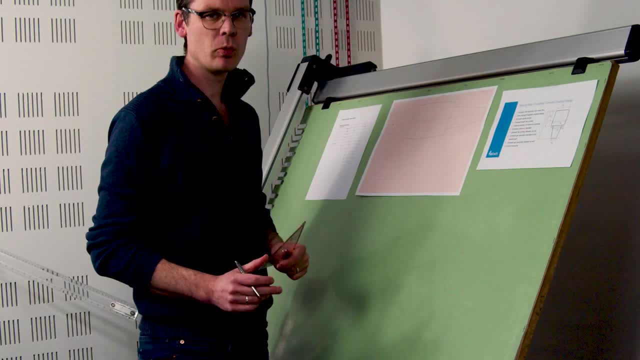 finalizes the the cowling design of the turbo fan in terms of the side view, or turbo fan in terms of the side view, or turbo fan in terms of the side view or the top view. if you will, what we're now, the top view. if you will, what we're now. 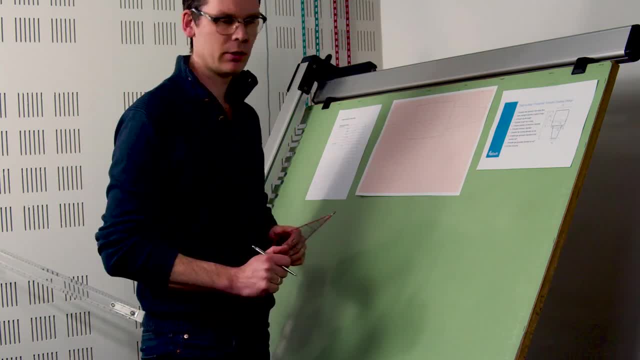 the top view, if you will. what we're now doing is we're focusing on on the front doing is we're focusing on on the front doing is we're focusing on on the front view and withdrawing in the front view view and withdrawing in the front view. 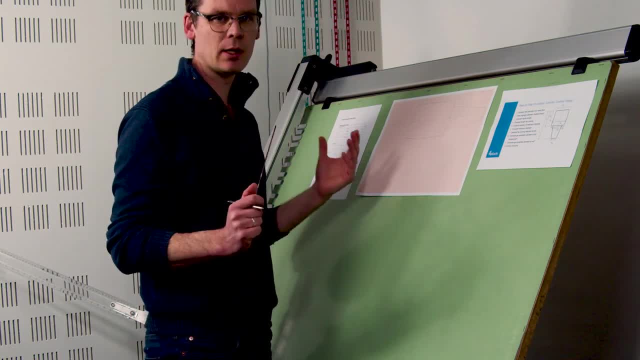 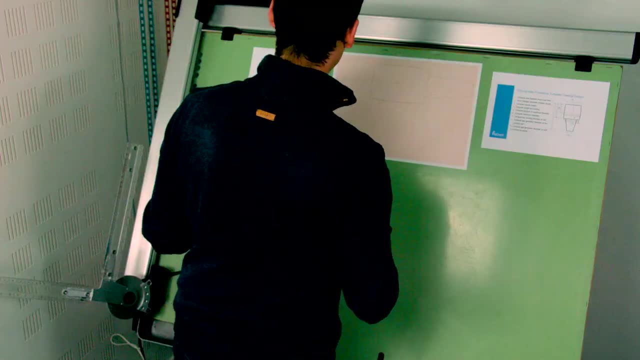 view and withdrawing in the front view, for that first thing that we're doing is for that first thing that we're doing is for that first thing that we're doing is: we're drawing the, the, the outermost. we're drawing the, the the outermost. we're drawing the, the the outermost diameter. so I get my geometric compass. 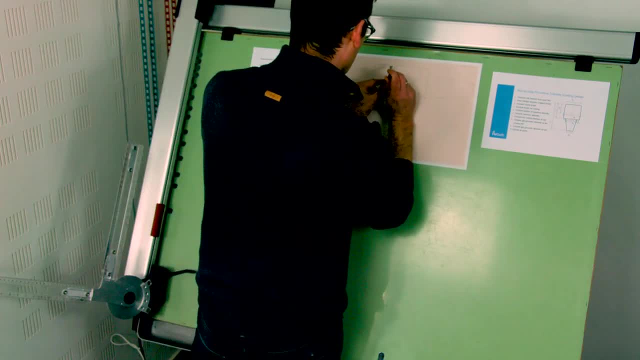 diameter, so I get my geometric compass diameter. so I get my geometric compass here and I can either look at, look at here and I can either look at, look at here and I can either look at, look at the datasheet or just look at the line, the datasheet, or just look at the line. 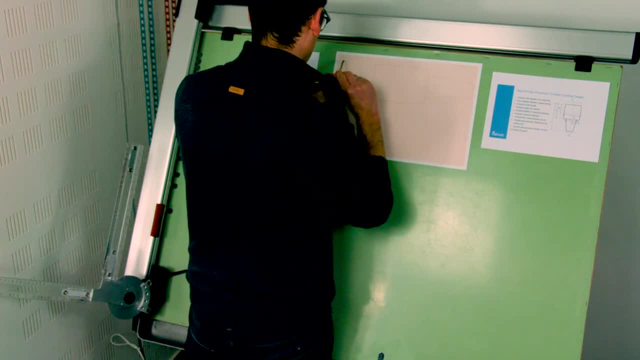 the datasheet. or just look at the line that I did before. make sure I got the that I did before. make sure I got the that I did before. make sure I got the same diameter from the side view. draw same diameter from the side view. draw same diameter from the side view. draw that in. all right, so that's the. 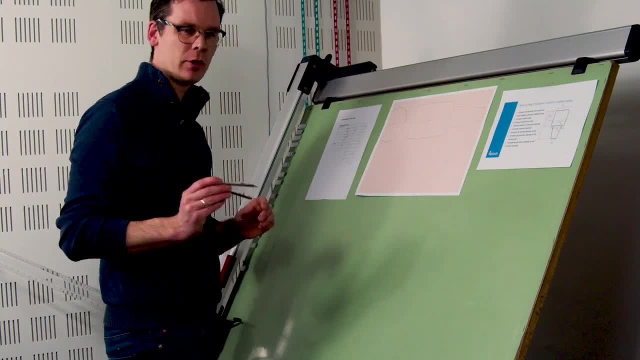 that in all right. so that's the. that in all right. so that's the outermost diameter. okay, so the next outermost diameter, okay, so the next outermost diameter, okay. so the next thing we're going to do is draw in. the thing we're going to do is draw in the. 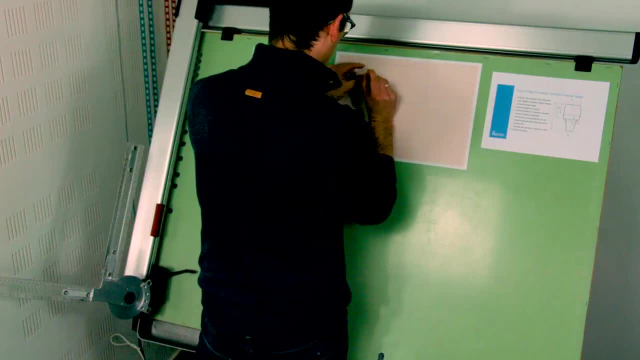 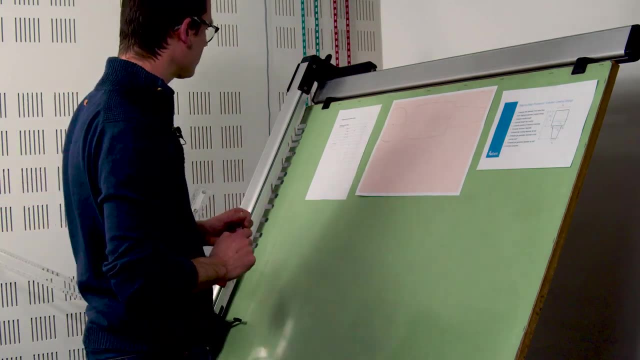 thing we're going to do is draw in the the inlet diameter. we're gonna start the inlet diameter. we're gonna start the inlet diameter. we're gonna start here. and the final thing I want to do here, and the final thing I want to do here, and the final thing I want to do is draw in the spinner and I computed. is draw in the spinner and I computed is draw in the spinner and I computed the spinner with the spinner to inlet the spinner with the spinner to inlet the spinner with the spinner to inlet ratio, which is point 18 which we ratio, which is point 18 which we.